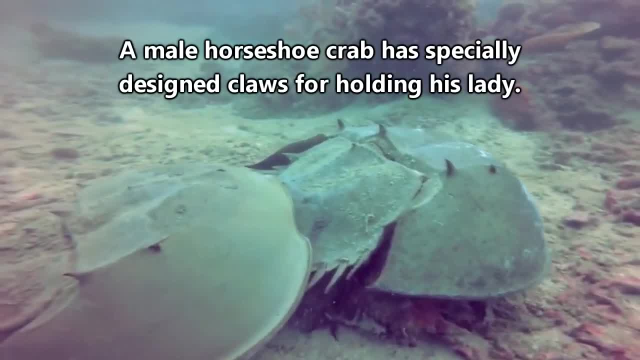 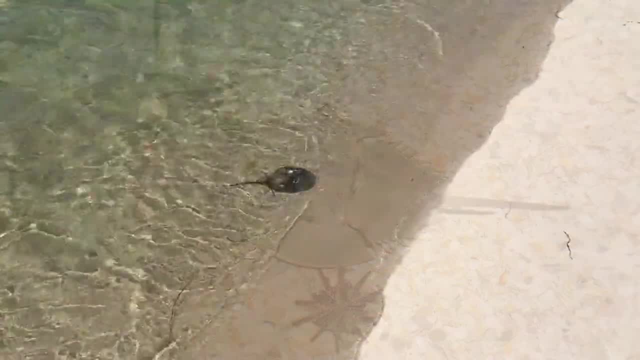 male clamoring for a female's attentions, and a male will go so far as to hold onto the female and ride on her back to her nest Freeloaders. Once finished, usually before the break of morning, all the adult horseshoe crabs will. return to the water, leaving their eggs defenseless. The horseshoe crab babies that will be able to survive the onslaught of predators that will then ensue will hatch a few weeks later. They'll molt as they grow to become adult-sized, which can be lengths of more than two feet with females. 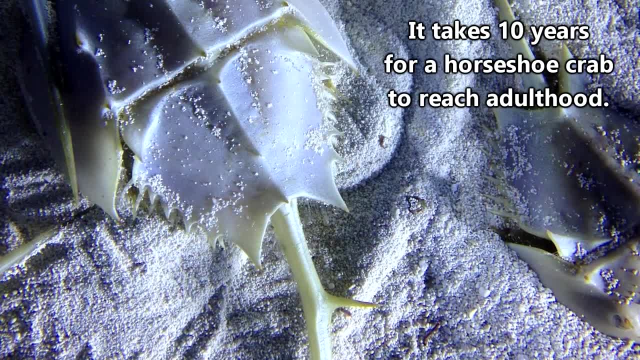 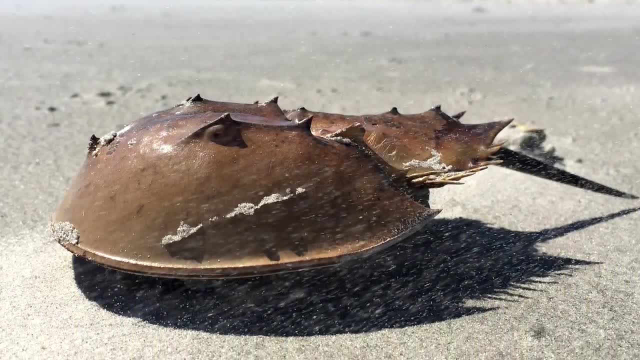 appearing larger than males. Horseshoe crab juveniles will molt approximately 16 times in the 10 years before they reach adulthood. During their lifetime, horseshoe crabs enjoy meals of worms and mollusks such as clams. 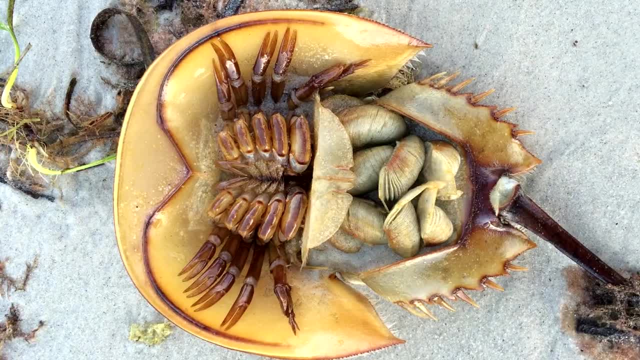 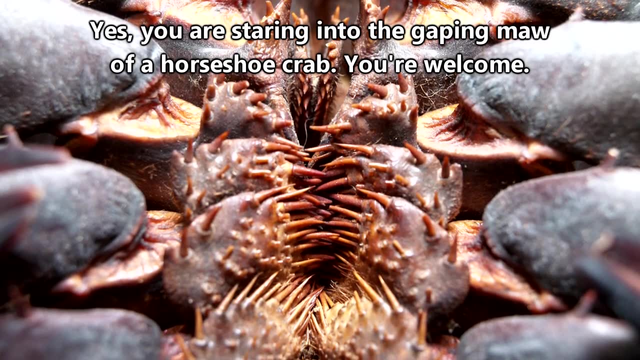 as well as dead fish. They chew their food with their feet, since they don't have any teeth. Yeah, their feet, no joke. They'll tear the food into small bits which can more easily fit into their mouths, which are located between their legs. Horseshoe crabs can live to be. 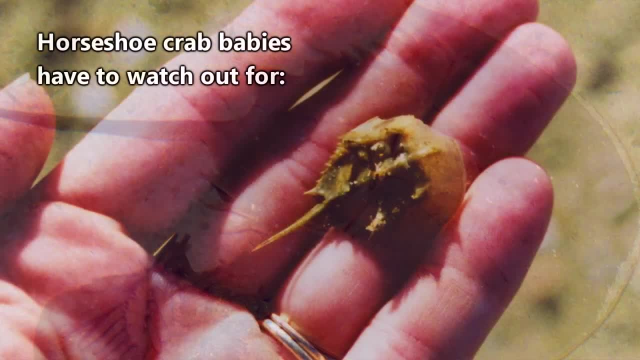 more than 20 years old, so long as they can avoid predators. As eggs and juveniles, horseshoe crabs are consumed in large quantities by shorebirds, crustaceans and other animals. Horseshoe crabs are also known for their long, long legs. Horseshoe crabs are also known. 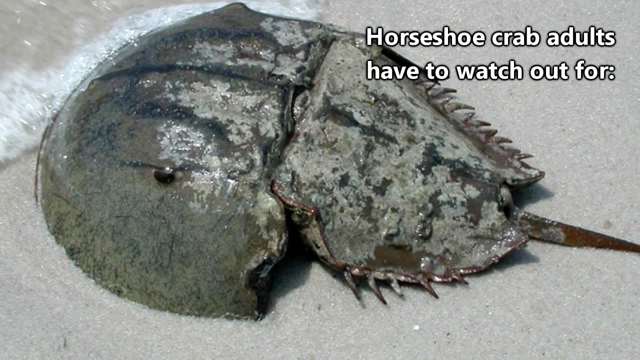 for their long, long legs. Horseshoe crabs are also known for their long, long legs. Horseshoe crabs are thought to eat large amounts of fish and fish intestines. As adults, horseshoe crabs face persecution from raccoons, foxes, sea turtles, alligators and humans. 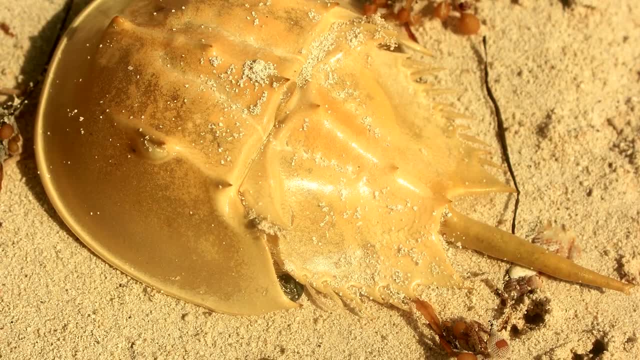 There are several reasons why horseshoe crabs are called horseshoe crabs, and we also use them for their blood daily. Horseshoe crabs have a special clotting agent in their blood that is used to make LAL or 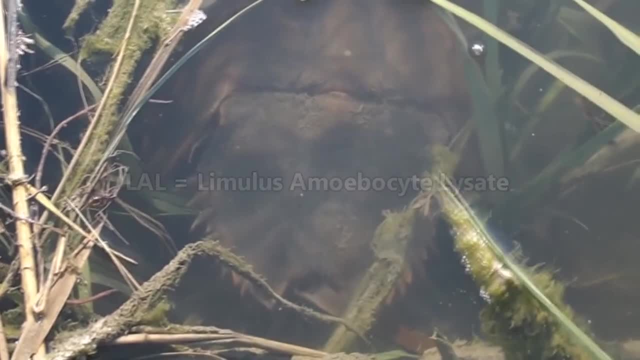 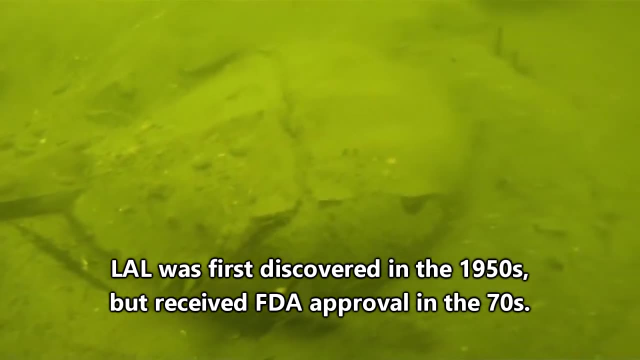 aircraft loads that are掰掰. LAL is a substance that is able to detect what are called gram negative bacteria such as E coli. Since the 1970s, LAL has been used in the medical industry to assess możlobs, because the tons of it can revealância of Negro. 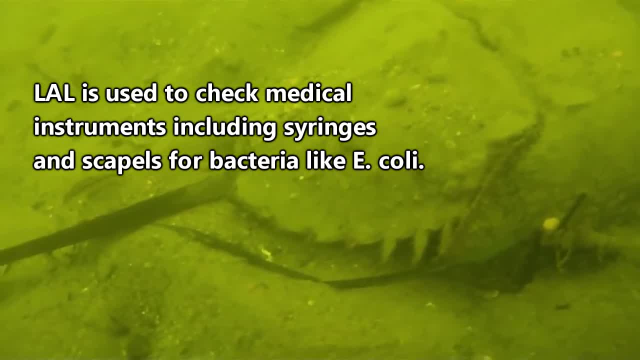 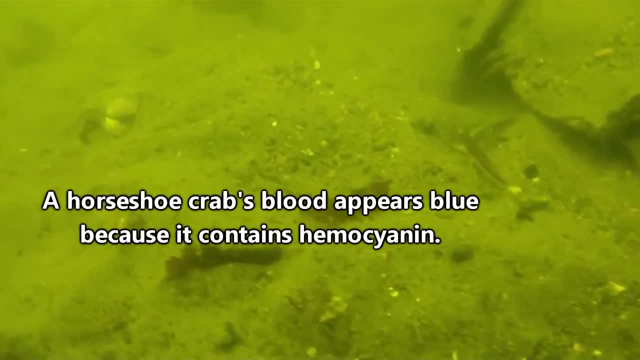 usted by men for gram-negative bacteria, which means it's possible that horseshoe crabs have saved your life. Unfortunately, the only way to produce LAL is to harvest blue-colored blood directly from horseshoe crabs. Horseshoe crabs are caught and brought to labs, where approximately one-third of their 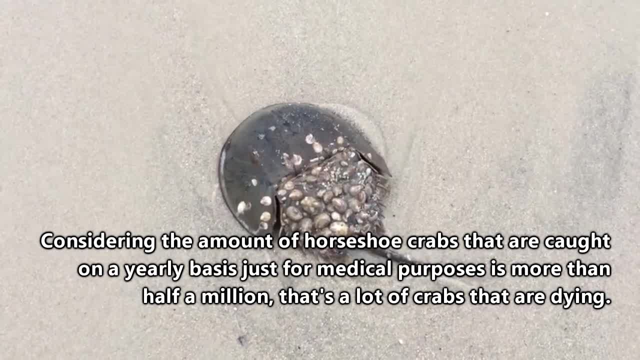 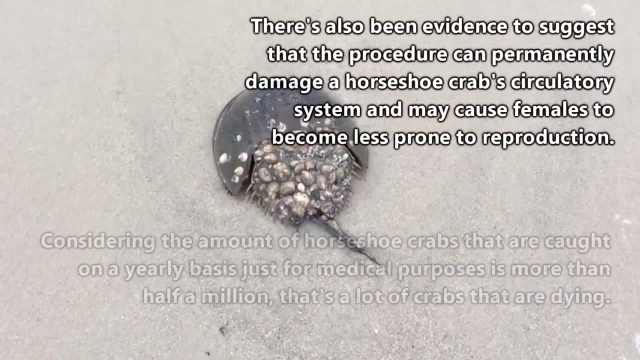 blood is extracted, at which point they are released back into the wild. It was once believed that this process was not detrimental to the individual horseshoe crabs being caught or to the general horseshoe crab populations, but recent research would suggest otherwise.